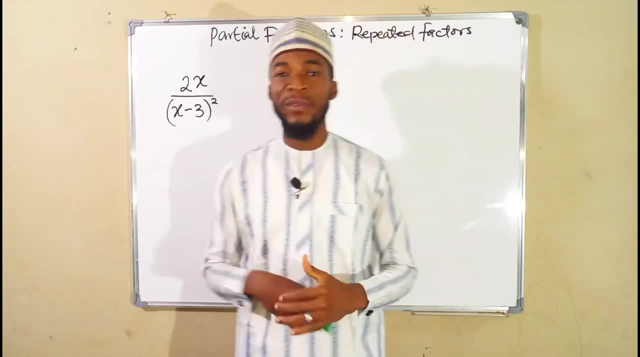 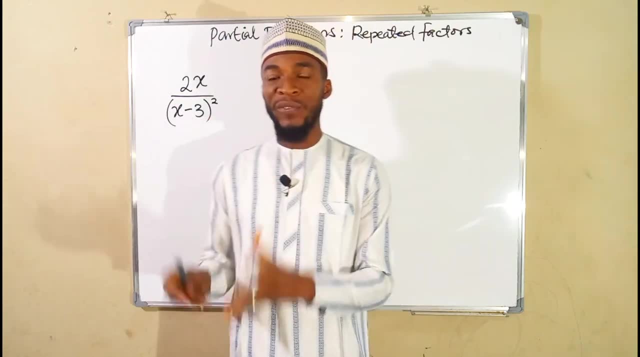 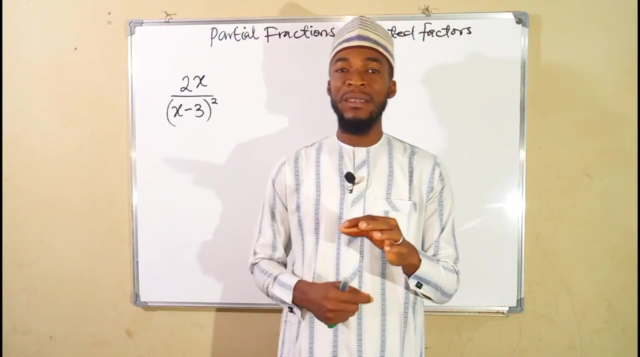 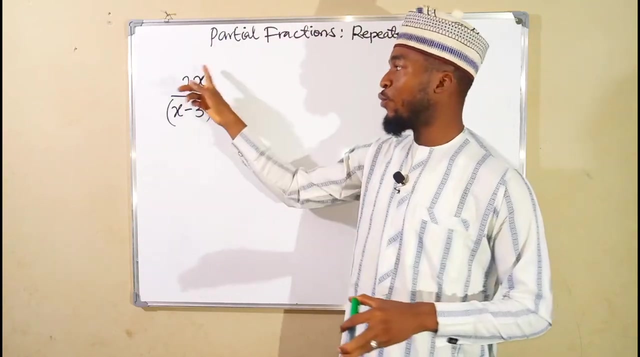 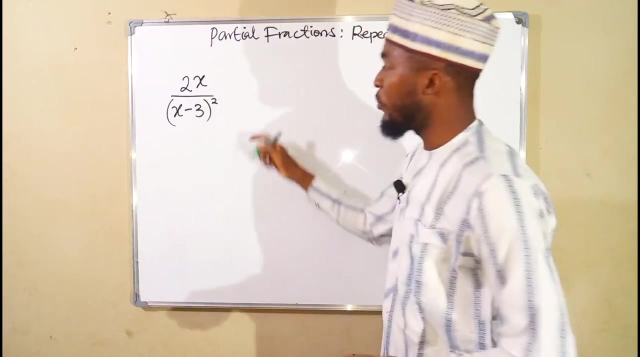 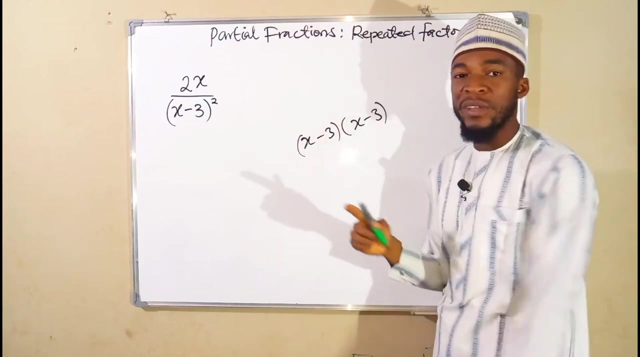 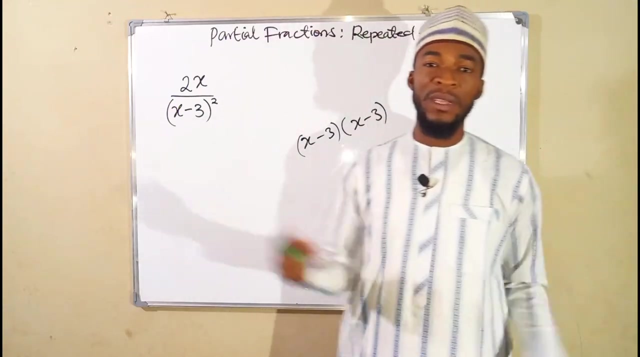 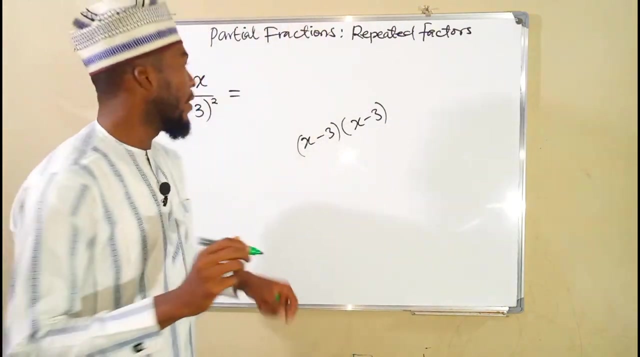 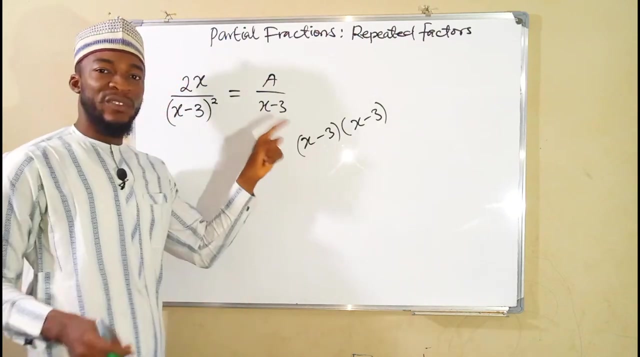 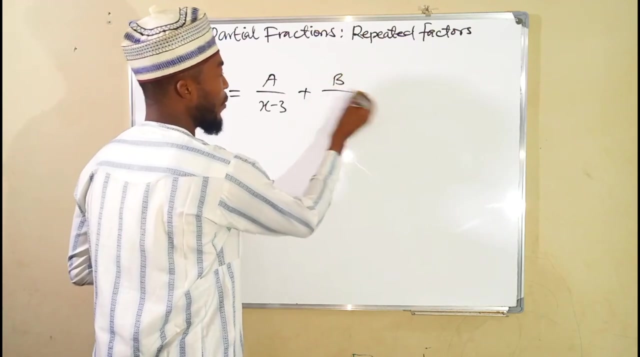 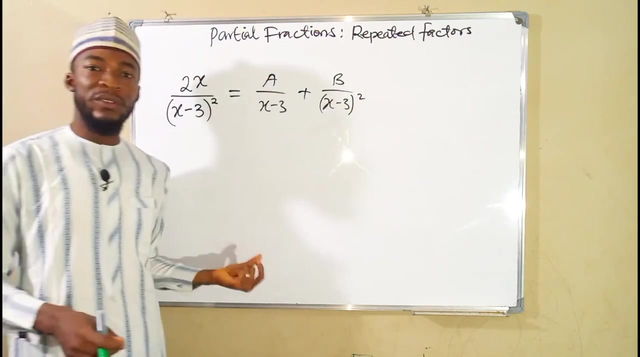 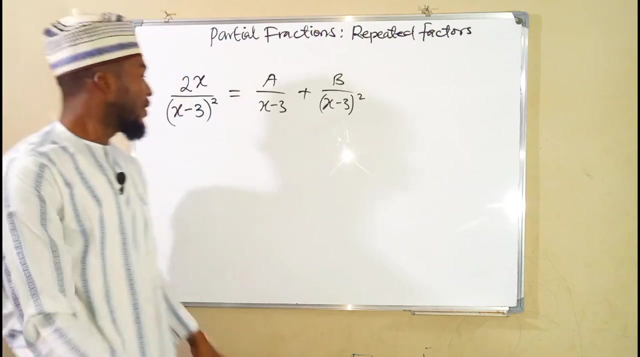 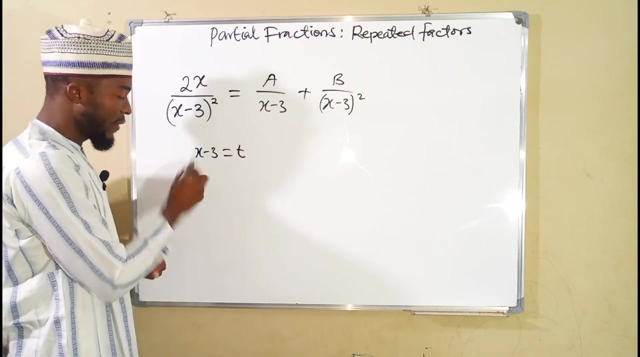 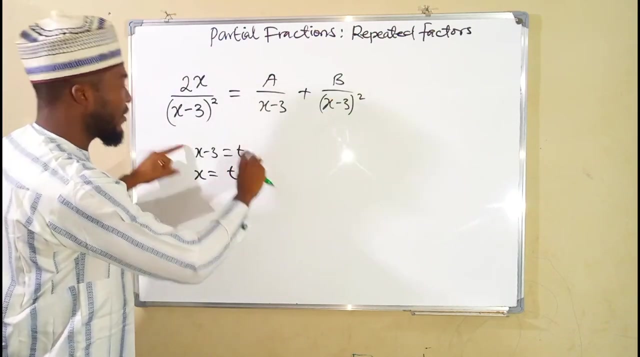 Hello good morning viewers. Still on to how to resolve compound fractions into partial fractions. Today I want to show you how to break down a compound fraction that contain a repeated factor. A repeated factor in the sense that the factor contain a power greater or equal to 2. For instance you can see in this first example we have 2x divided by x minus 3 to the power of 2. This x minus 3 to the power of 2 is the same thing as x minus 3 multiplied by x minus 3. You can see the two factors are exactly the same and hence we see they are repeated. And this power can be more than 2, 3, 4, 5 in that order. So let me show you how to break this down. This will be equal to some constant, let me call it a, over x minus 3 to the first power plus some constant, let me call it b, over x minus 3 to the second power. You know we have two factors and definitely we are going to obtain two fractions. But why do we split them in this form? I will show you why. Suppose this x minus 3 is equal to t. x minus 3 equals t. You can see x can now be equal to t plus 3. Now let us substitute this information back here. On the first one we are going to 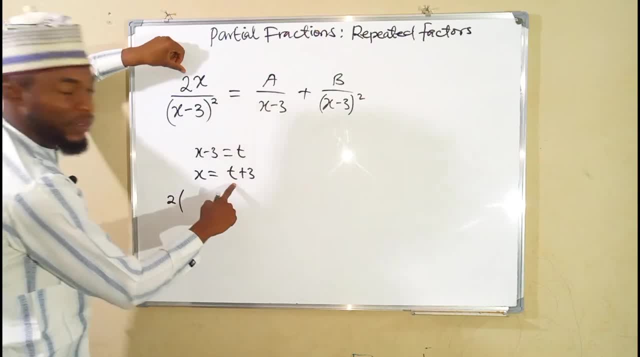 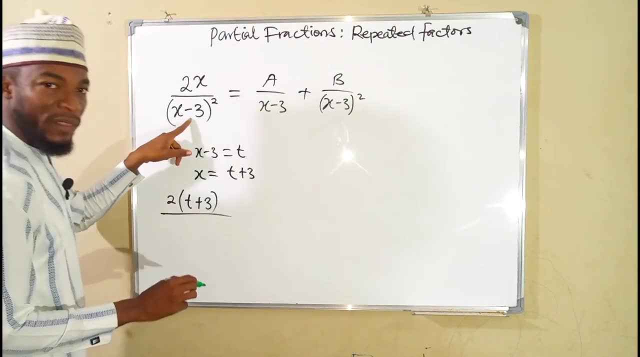 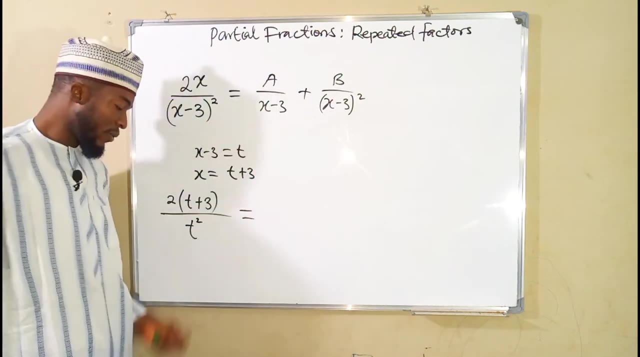 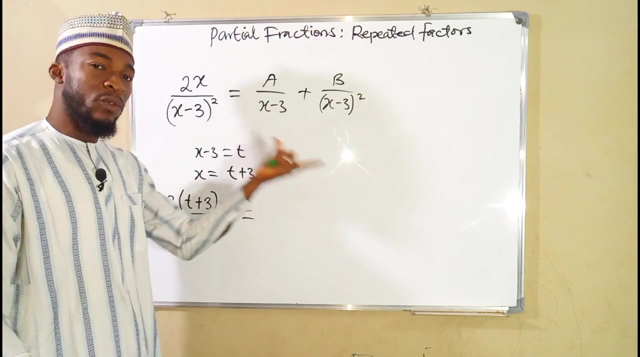 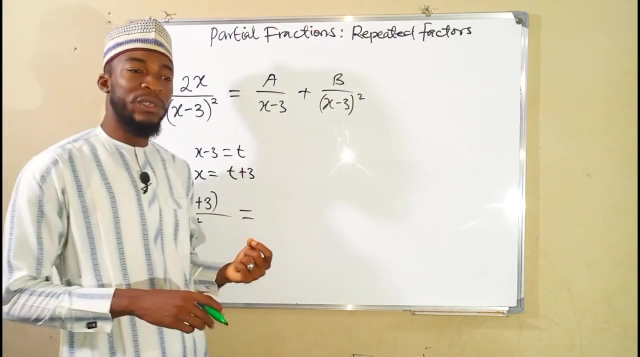 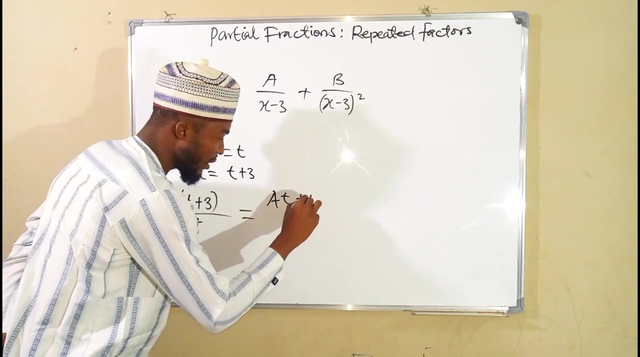 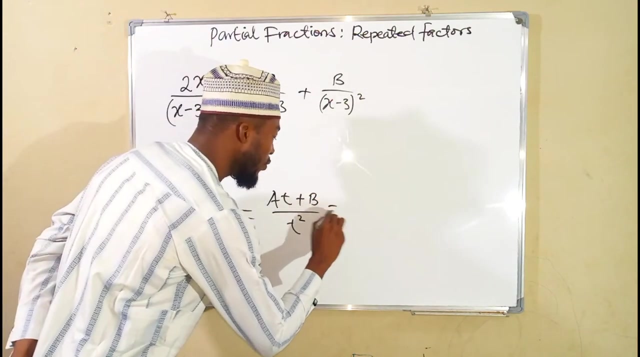 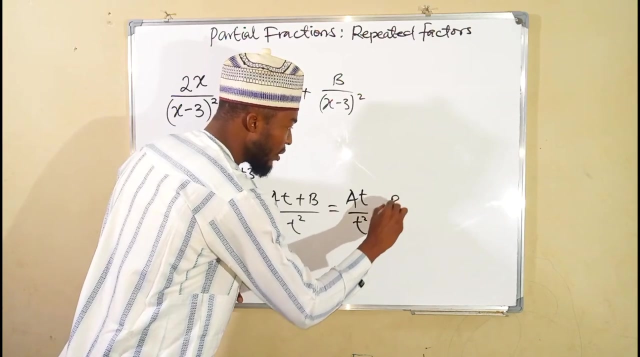 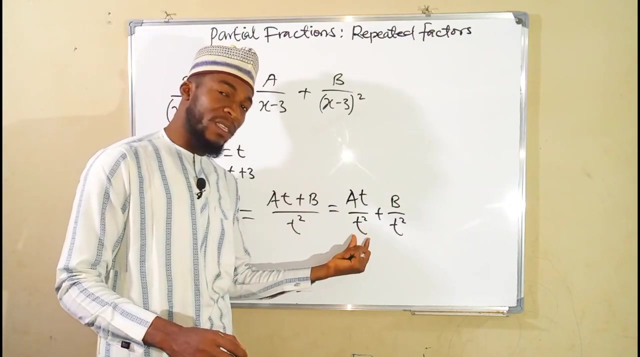 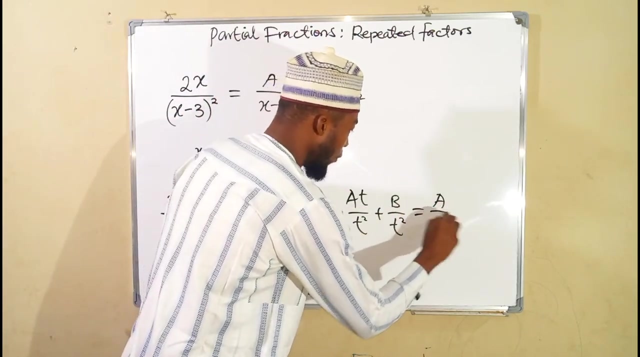 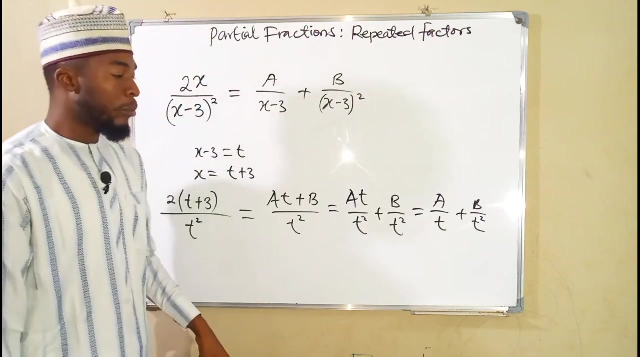 obtain 2 multiplied by x which is now t plus 3, divided by, we have already substituted this to be equal to t, to the second power. Let us dissolve this. You know this is a quadratic factor and I told you to split a quadratic factor into partial fraction. The numerator is always going to be a polynomial of one degree less than the denominator. So that polynomial is going to be a linear function. So we have a t plus b over t to the second power. And this can also be written as a t over t squared plus b over t squared. But from here we have t times t and we have a single t to the top. So one t can cancel the other, leaving only a over t plus b over t squared. 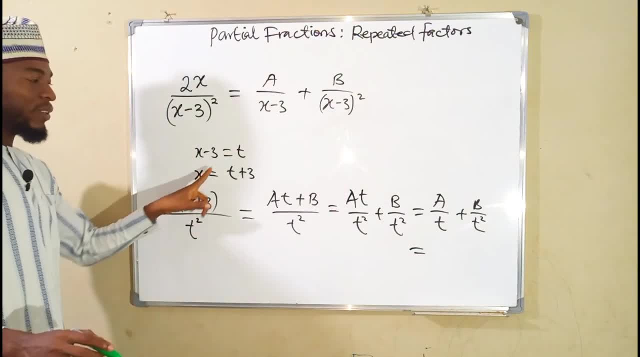 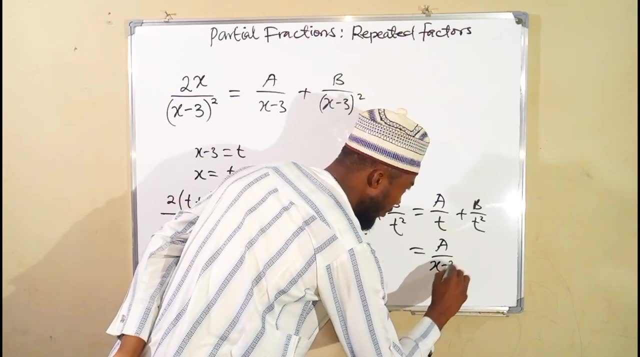 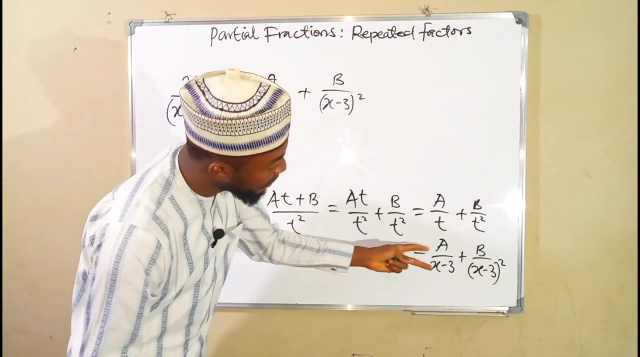 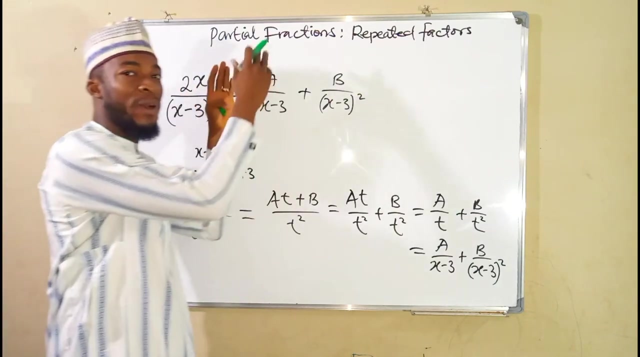 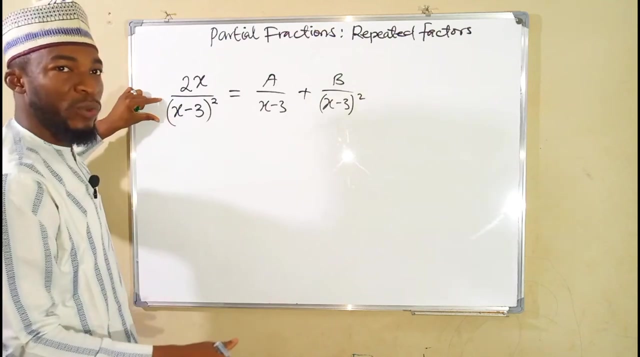 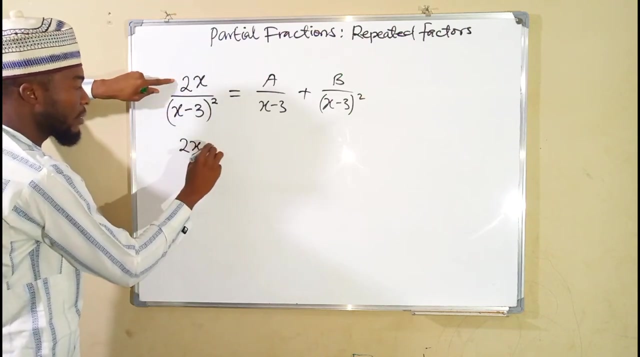 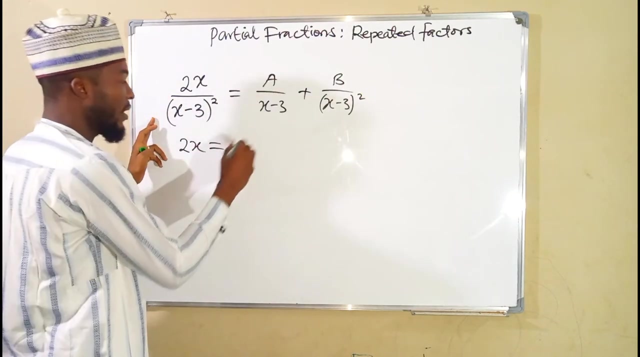 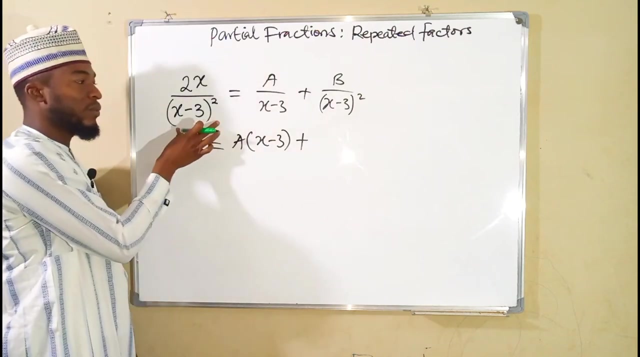 So remember, from here our t is equal to x minus 3, so we can say a over x minus 3 plus b over x minus 3 to the second power, and you can see these fractions are exactly as the initial ones. So this is why we dissolve our partial fraction in this form when we have the repeated factors. If we multiply each of these times by this factor x minus 3 to the second power, the first one is going to cancel this leaving only two x at the top. This is equal to multiply this by this factor, this would cancel one of the factor leaving one times a. So we have a multiplied by x minus 3 plus times this by this factor, they are exactly the same, they are going to cancel out leaving only b. 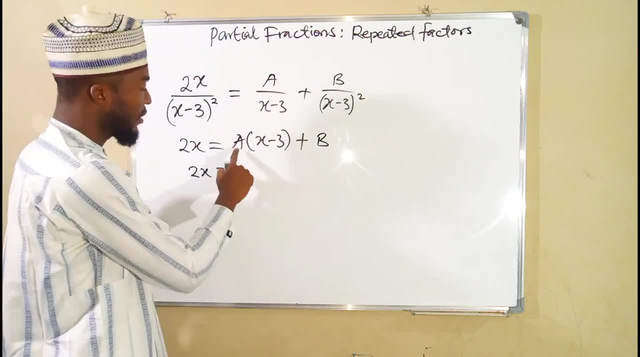 To do x to the left is equal to, you can now expand this, a times x is ax, a times negative 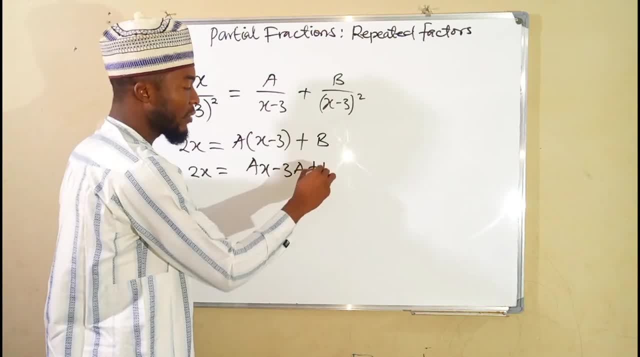 3 is negative 3a, then plus b. 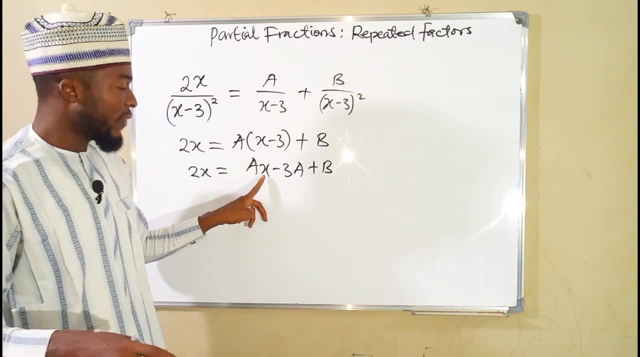 Now let us relate the coefficients. The coefficient of x to the right is just a, and the coefficient of x to the left is 2.